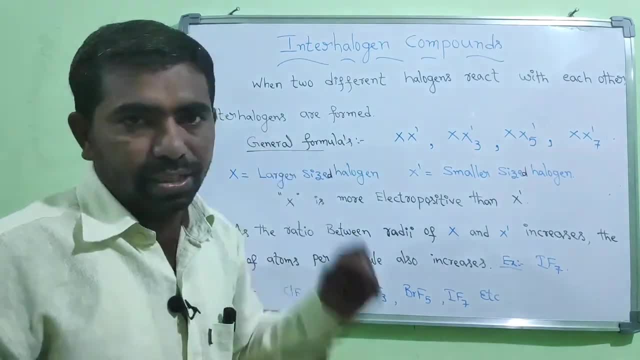 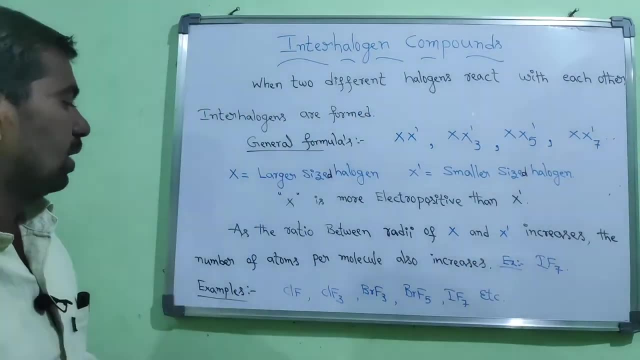 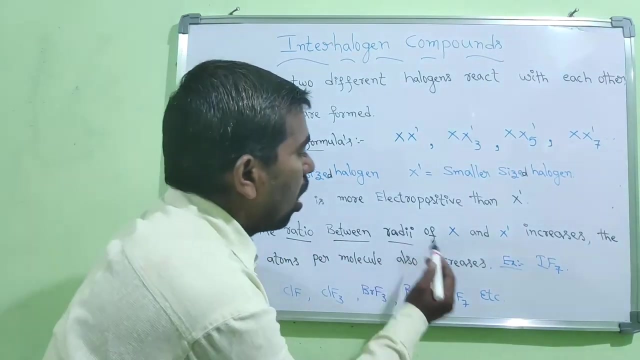 electronegativity is lesser than that of the x dash. x dash electronegativity is high, or the more So. that is about the x and x dash. So here one statement. I am saying So as the ratio between radii of x and x dash increases the number of atoms per molecule. 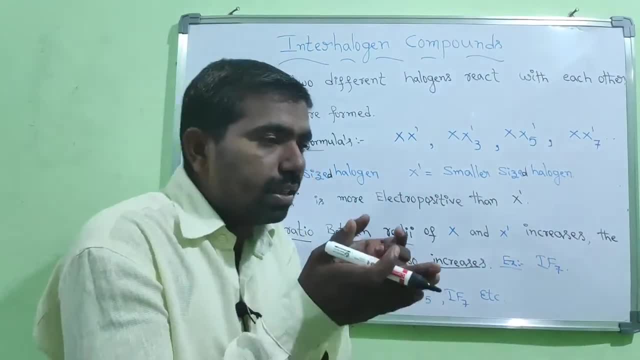 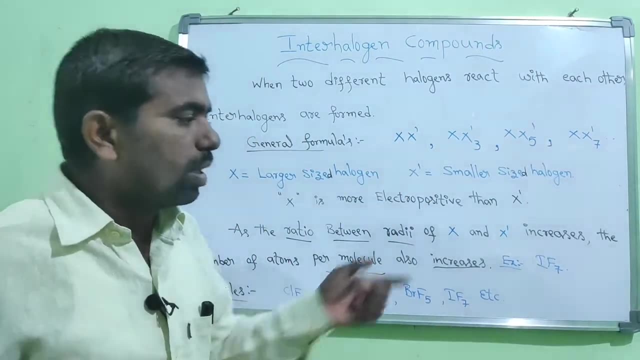 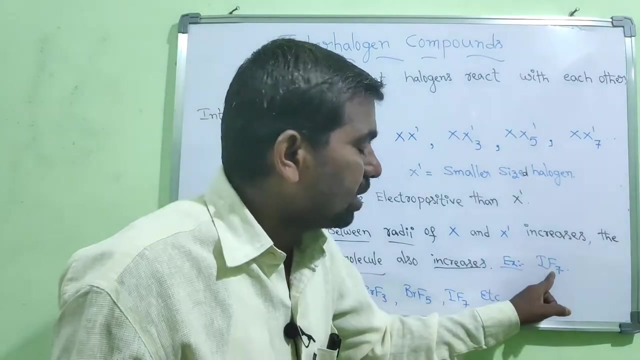 also increases. So when there is a more difference in the radius of x and x dash, so the number of atoms per molecule also increases. So for example, f7. Here the x is equals to i, x dash is equals to f. That means fluorine. So there is a large 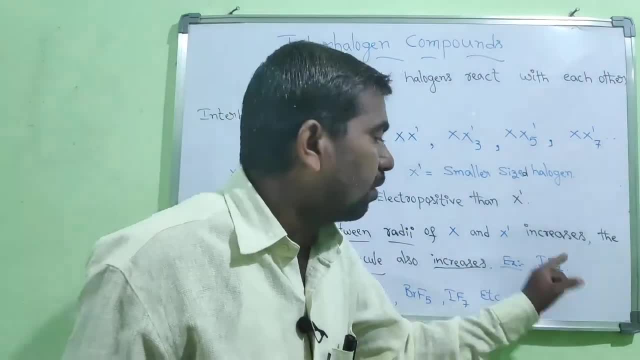 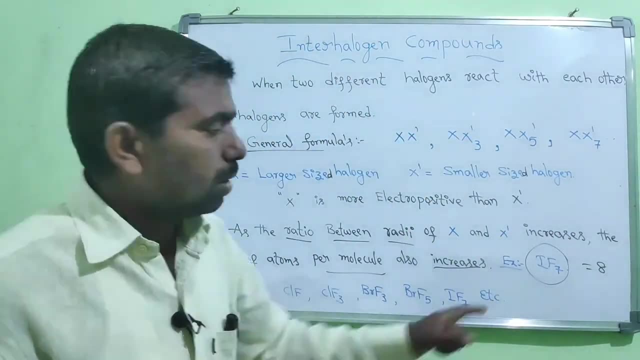 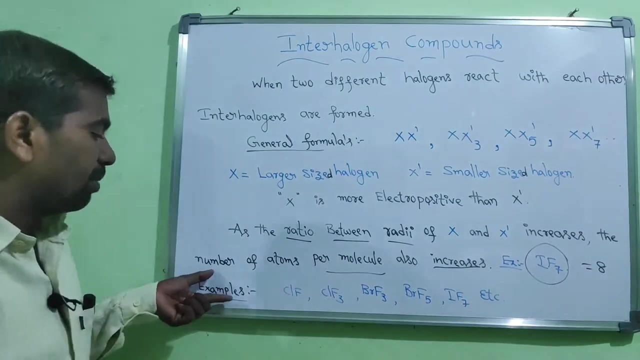 variation in the radius of iodine and the fluorine. So that is why the total number of atoms here eight atoms are there per molecule, So that means more number of atoms are existing per molecule. So that is about to this statement, And here I am giving some examples for the 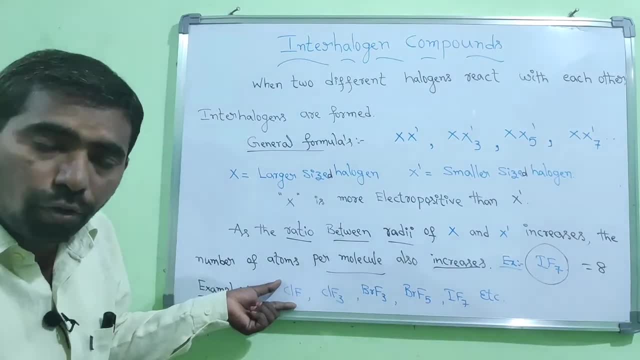 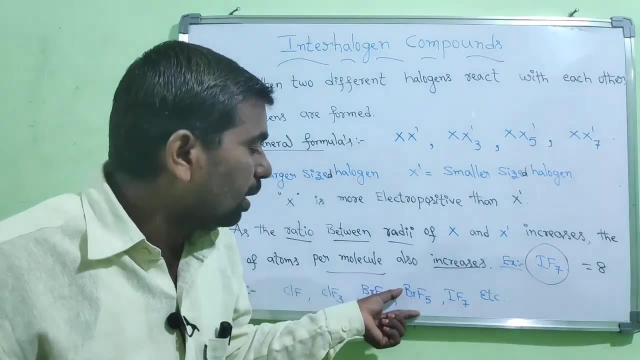 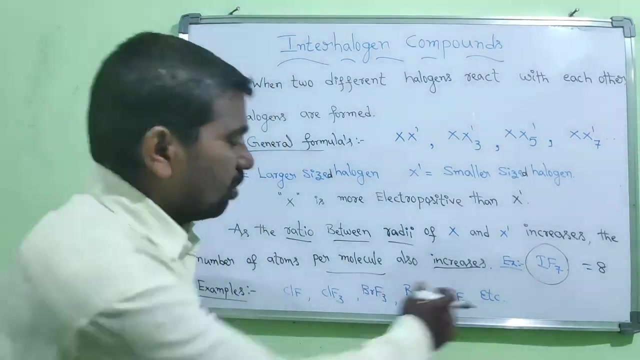 interhalogen compounds: CLF, Chlorine, fluoride, chlorine trifluoride, CLF3, BRF3, bromine trifluoride, BRF5, bromine pentafluoride, IF7, iodine heptafluoride, So, etc. These are the some of the examples for the 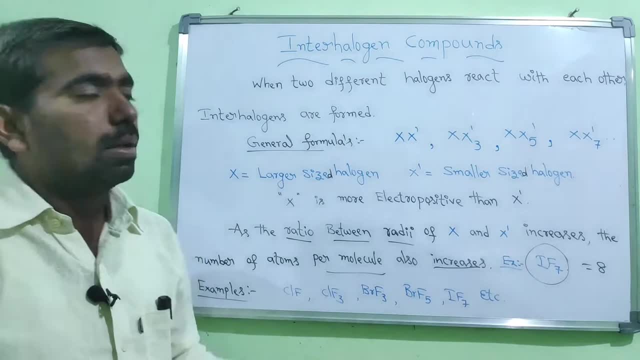 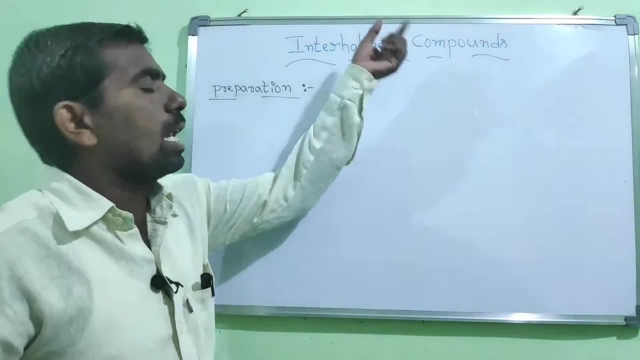 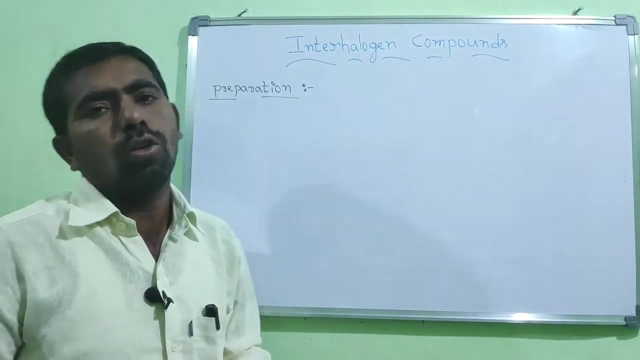 interhalogen compounds. Now we will discuss about the preparation of interhalogen compounds and some of the properties and their structures. Now the preparation of interhalogen compounds: The interhalogen compounds can be prepared by the direct combination of halogens. So 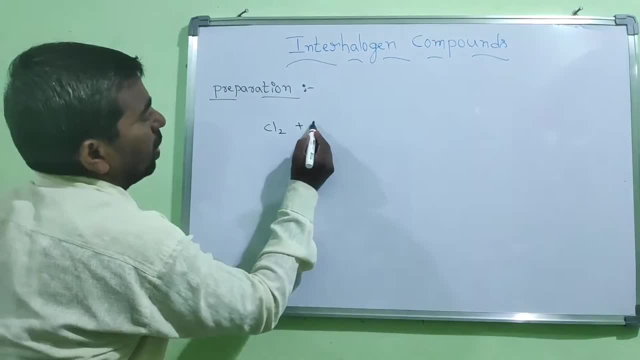 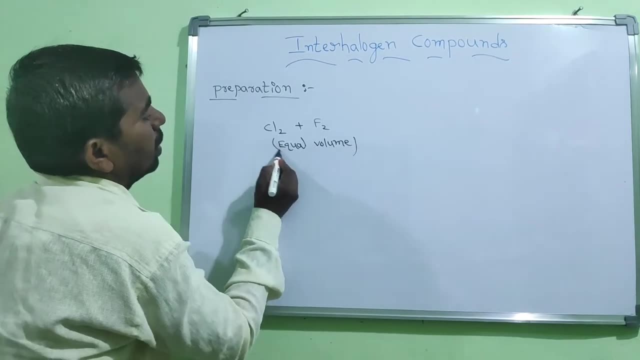 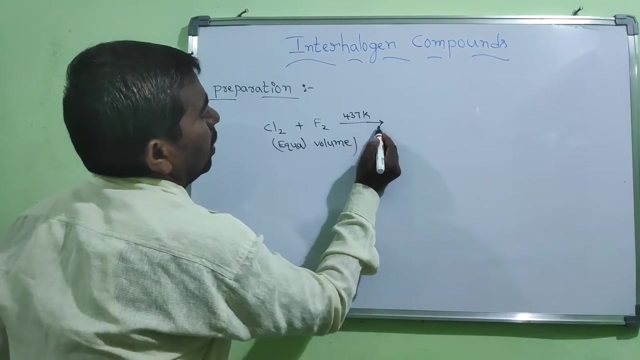 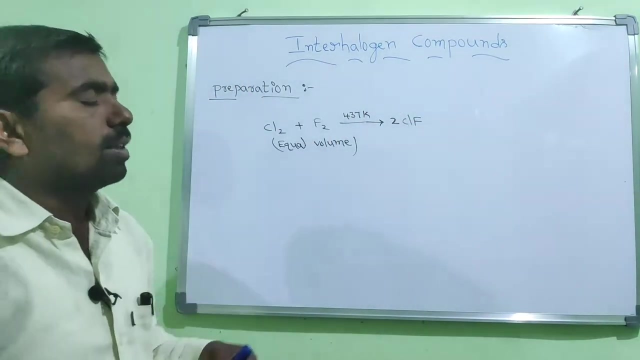 for example Cl2, chlorine molecule. I have taken F2. So these two are taken in a equal volume and provided certain temperature- 437 Kelvin, 2 ClF, Chlorine, fluoride, chlorine trifluoride- one of the interhalogen compound is obtained. So, for example, another, I am taking Cl2 plus. 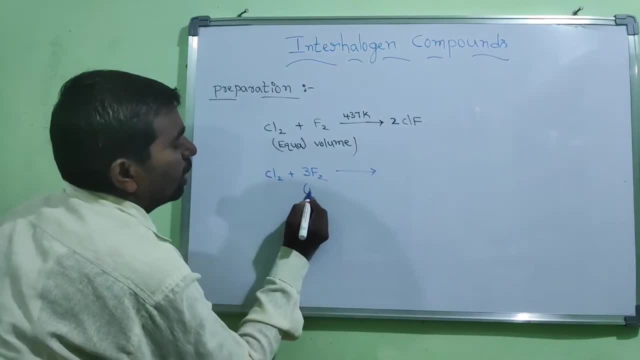 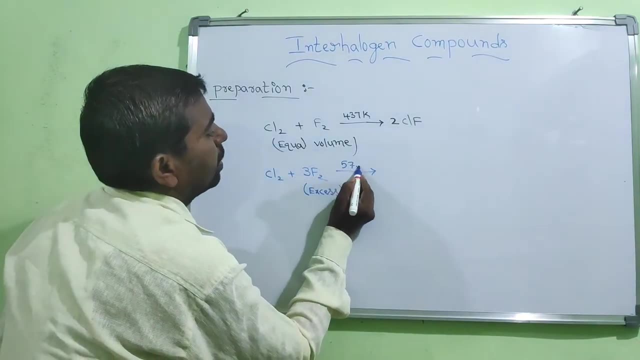 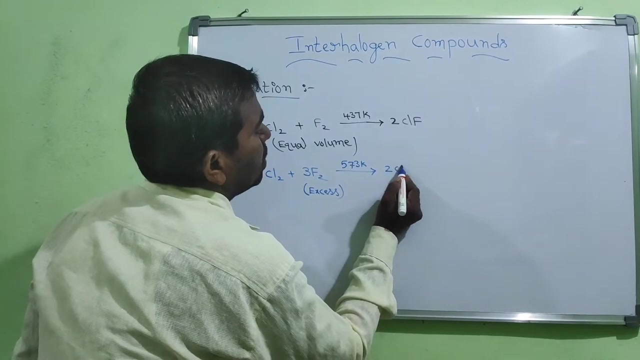 3F2.. So here fluorine I am taken. excess quantity, 573 Kelvin of temperature is provided for the reaction occurring in between these two: 2 ClF3.. Chlorine trifluoride is the product Chlorine fluoride. 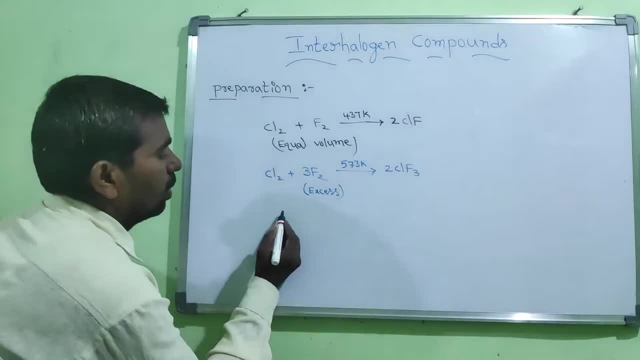 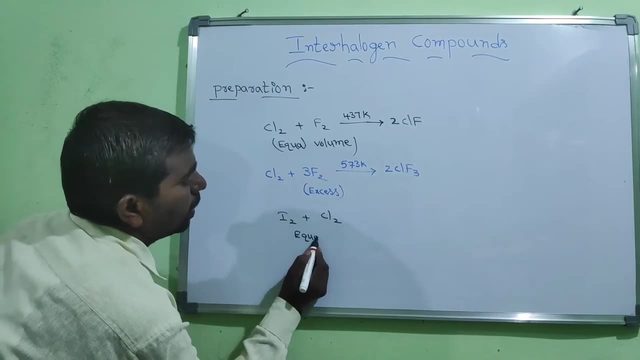 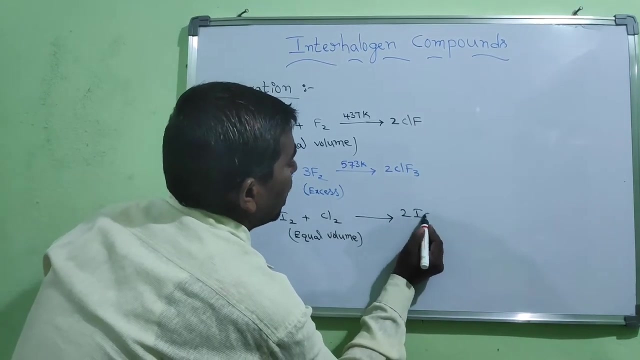 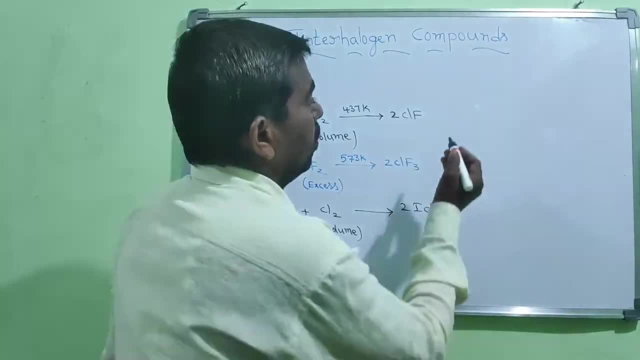 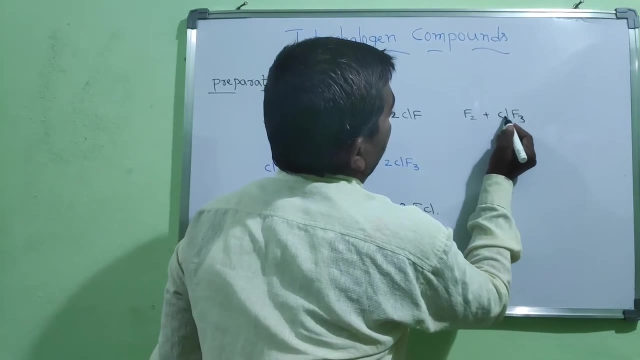 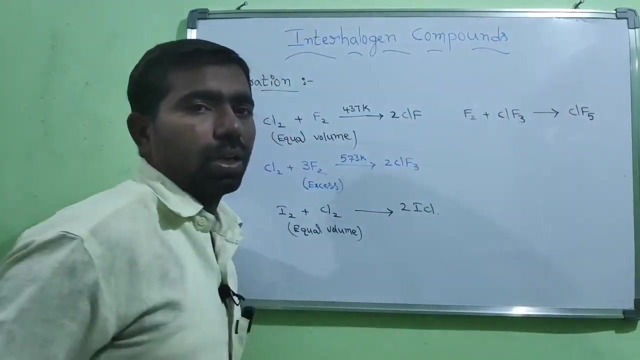 about the formation of iodine chloride, Another preparation I am doing, so fluorine I am taken. To this ClF3 is added Chlorine trifluoride. They are reacting with each other So formation of ClF5, chlorine pentafluoride is occurring. 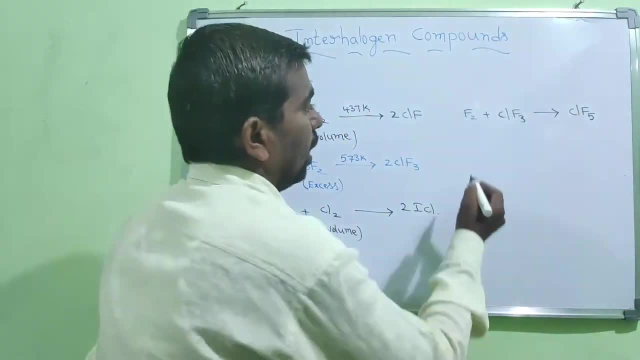 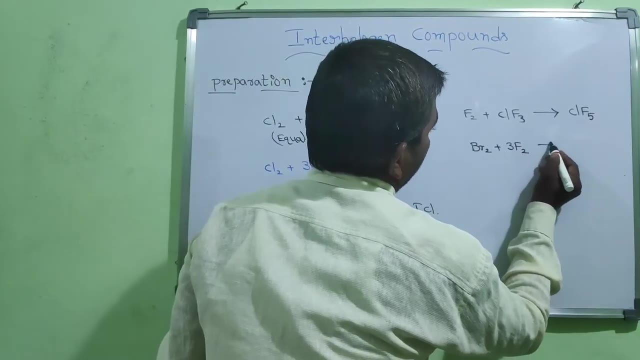 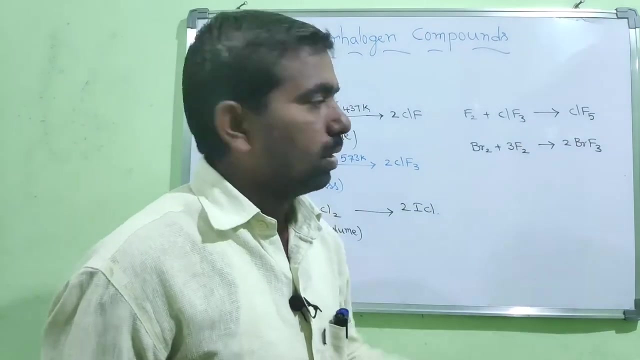 That is about the preparation of ClF5.. And another one I am giving as example: Br2 plus 3F2 gives us to 2BrF3.. So boron trifluoride is an interhalogen compound is obtaining in this chemical reaction. 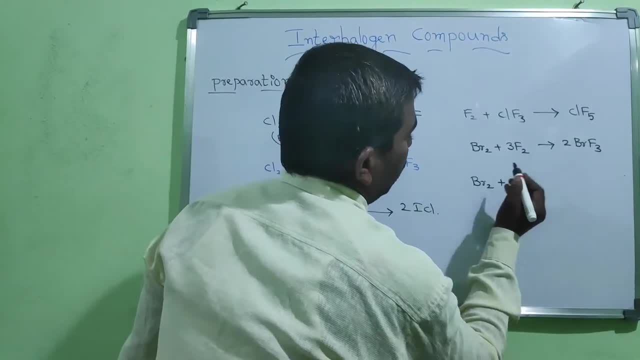 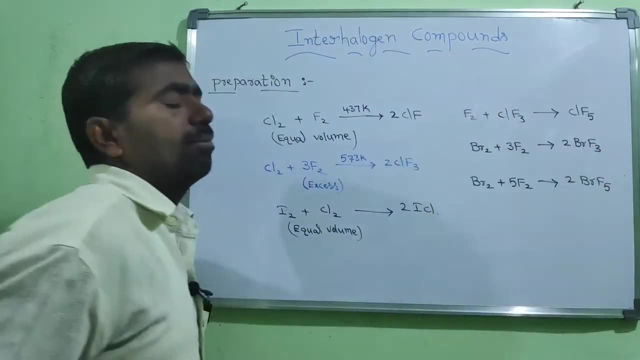 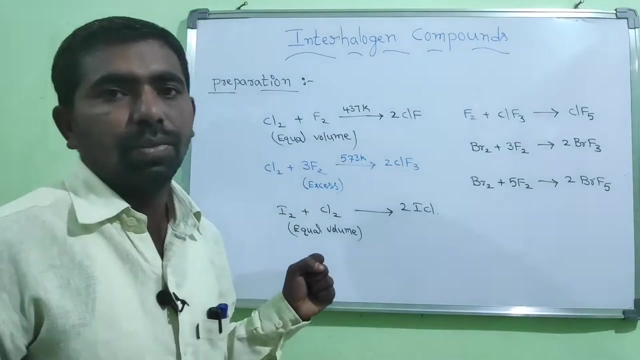 So another one I am giving as example: Br2 plus 5F2 gives us to 2BrF5.. So boron pentafluoride is the interhalogen compound is obtaining. So these are the some of the preparations for interhalogen compounds. 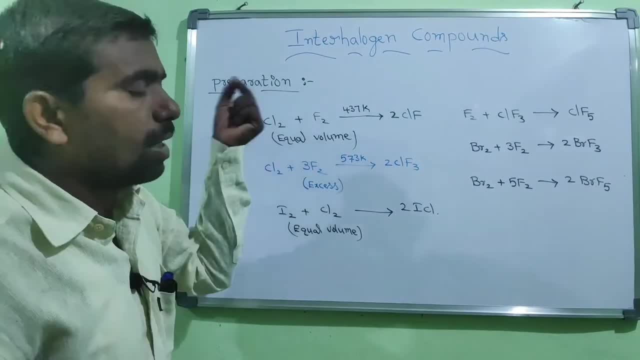 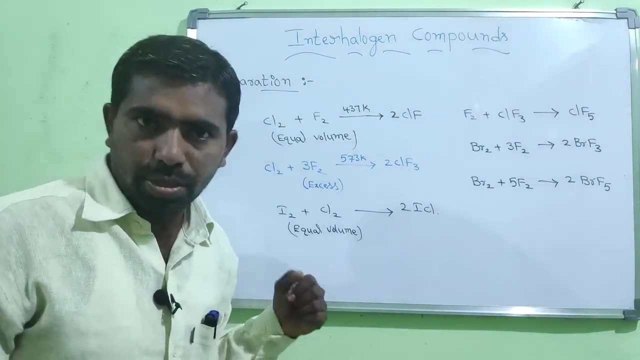 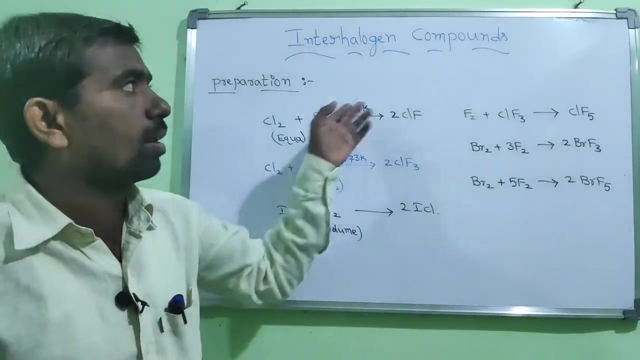 So in these preparations- so we are taking the two different halogens directly combining In certain chemical reactions- we have to provide certain Temperatures for occurring of a chemical reactions for the formation of interhalogen compounds. So this is about the preparation of interhalogen compounds. 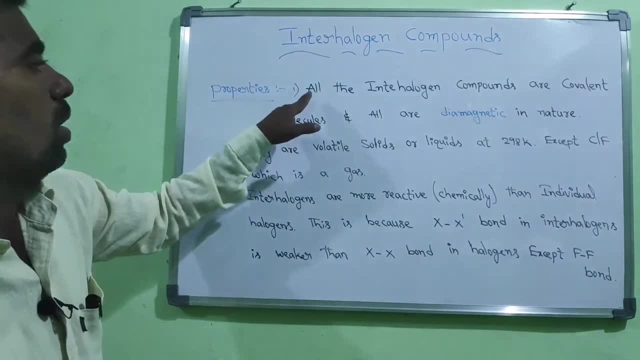 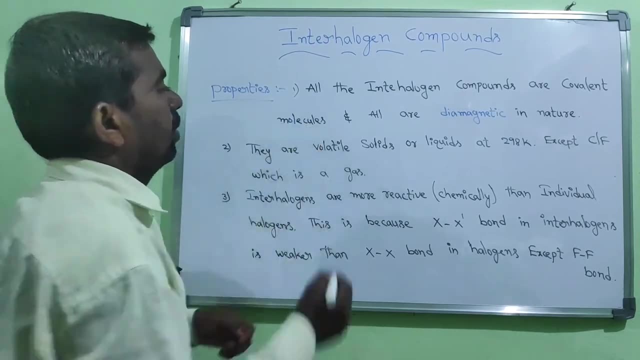 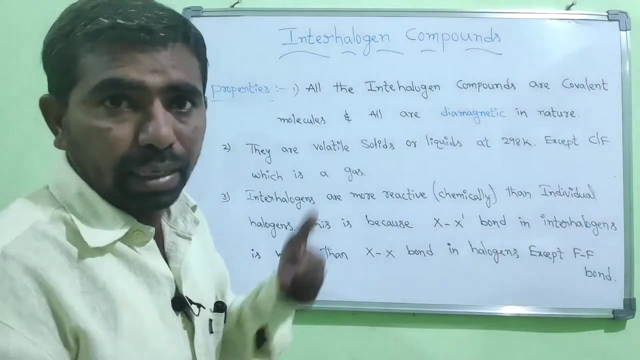 Now the properties of interhalogen compounds. All the interhalogen compounds are covalent molecules And all are diamagnetic in nature. So here magnetic property also said. So all are the diamagnetic in nature, They are volatile solids. 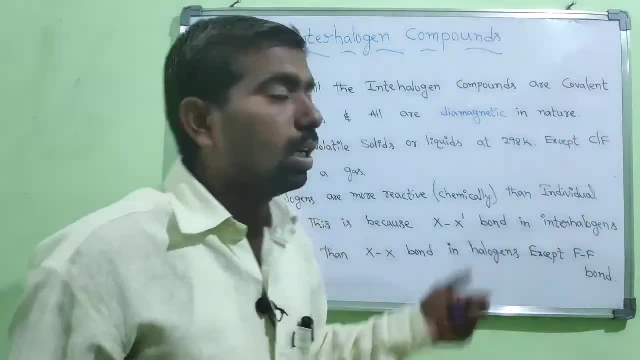 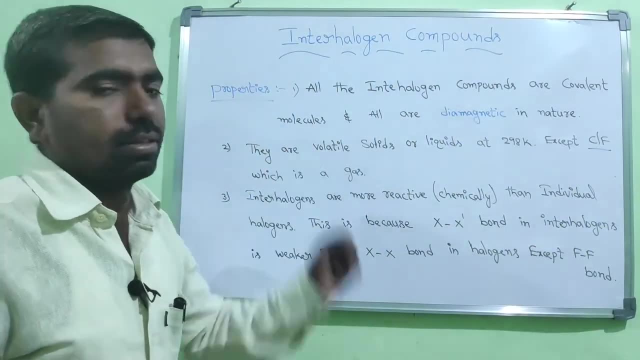 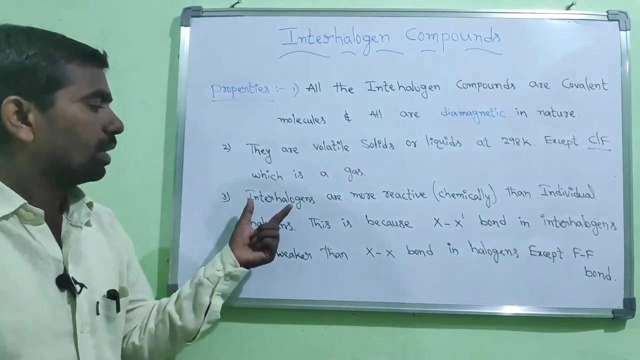 Or liquids at 298 Kelvin, That means at room temperature, Except chlorine fluoride. So chlorine fluoride, which is a gas, CLF is a gas, Except that one. all are volatile solids and liquids. Next property: interhalogens are more reactive chemically, I am said. 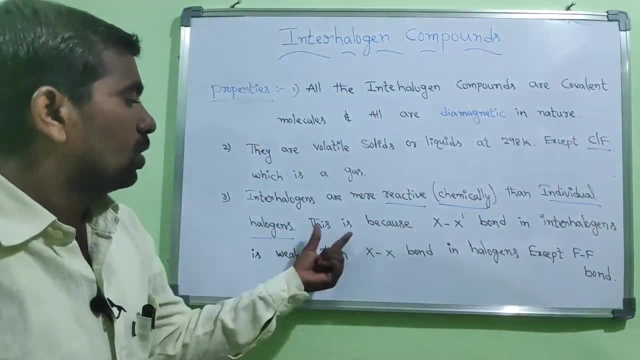 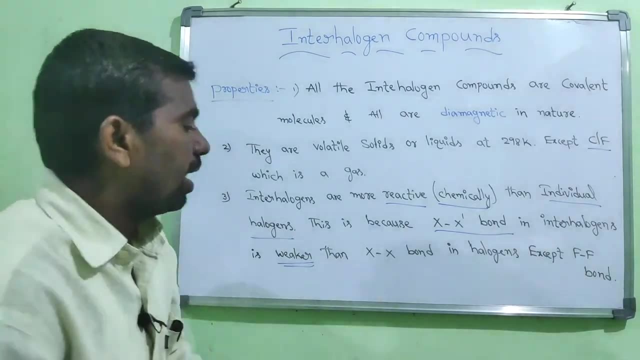 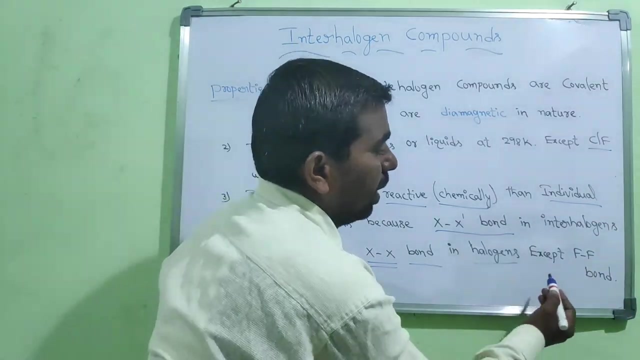 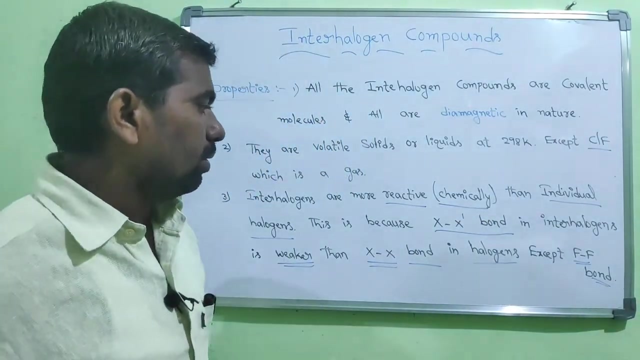 Than individual halogens. So this is because XCX dash bond In interhalogens is weaker than XCX bond, So individual halogen, So in halogens, except FF bond, That means FF bond is weaker than XCX dash bond. 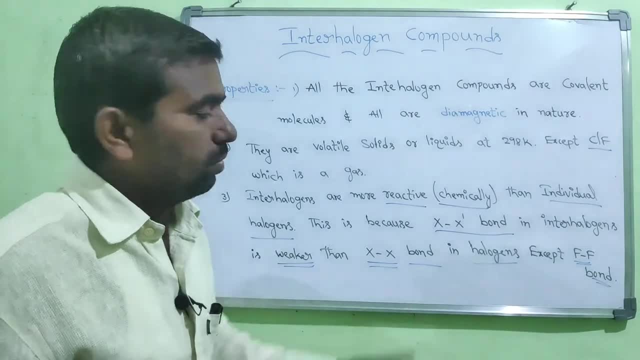 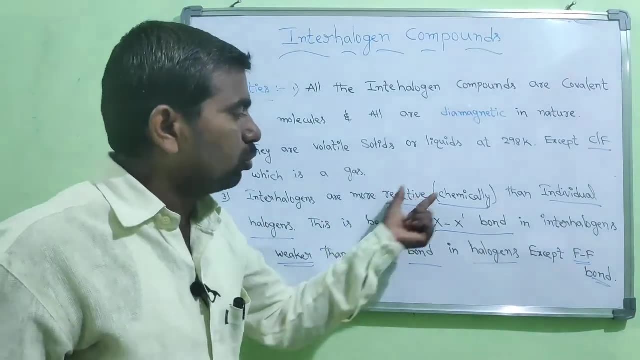 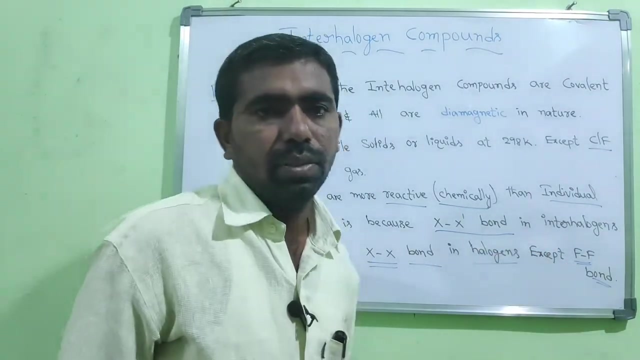 And XX bond is stronger than XX dash bond. So due to this, The interhalogens are more Reactive chemically Than the individual halogens, Except FF, That means fluoride. This is about some of the properties of interhalogens. 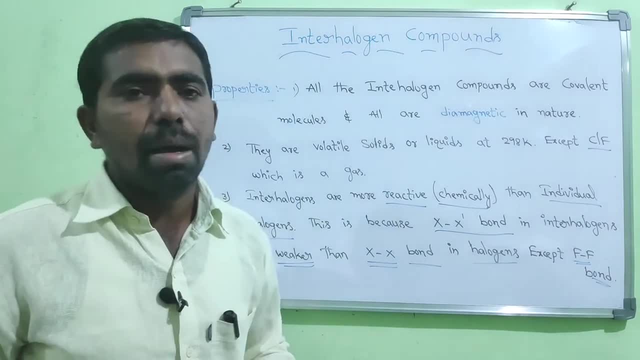 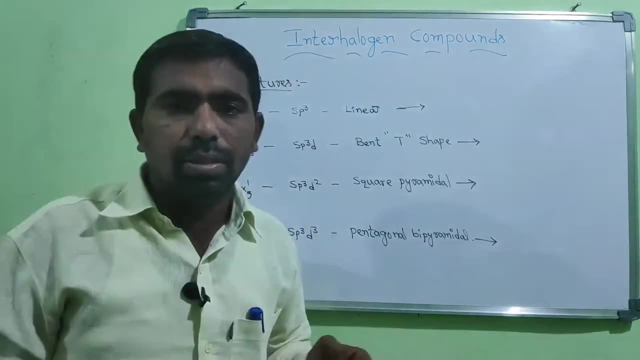 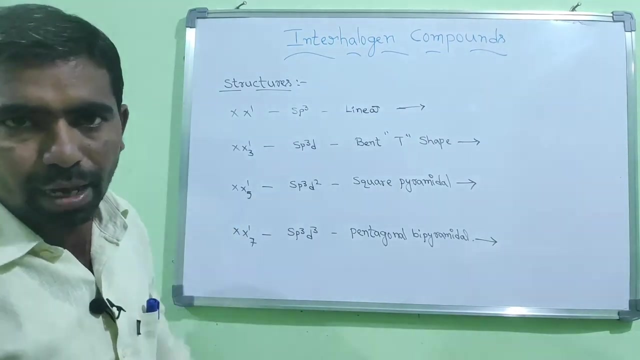 Now we will discuss about the structures Of these compounds, Now the structures of interhalogen compounds. Now I am explaining one of the shortcut method To explain the structures of these compounds. So, for example, I am taking any one of interhalogen compounds. 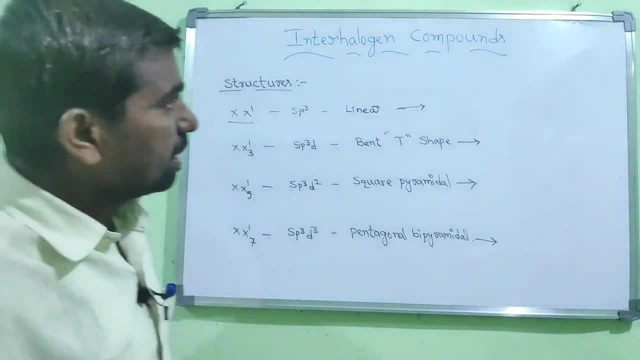 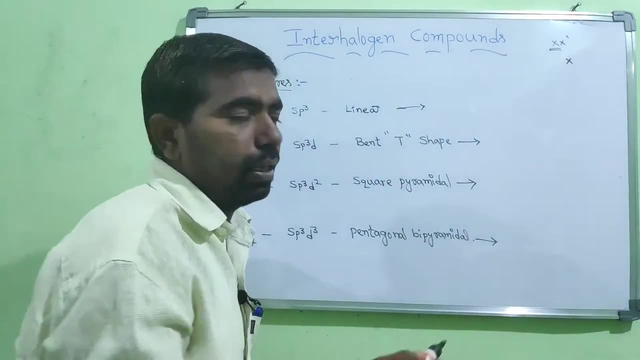 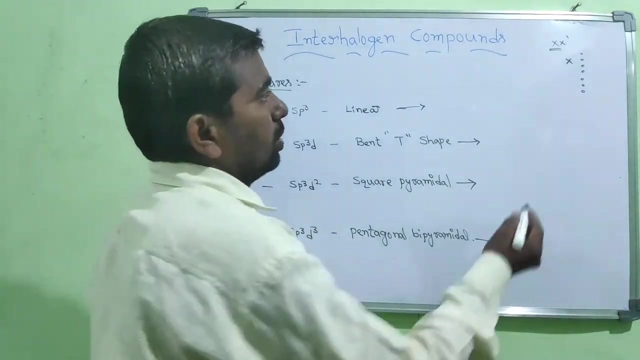 For example XX dash. In this molecule X is the central atom, So X belongs to halogen family. That means There are seven electrons In the outer sub. So XX dash, That is also halogen That has the ability to form only one single bond. 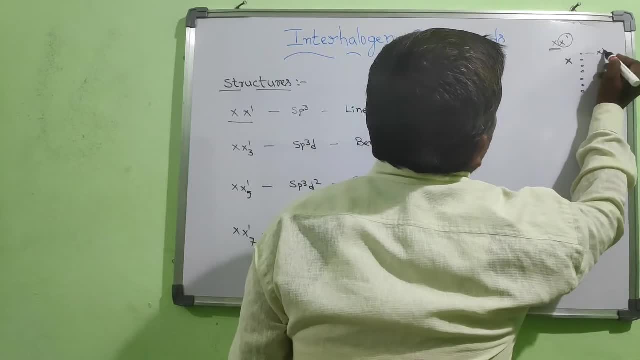 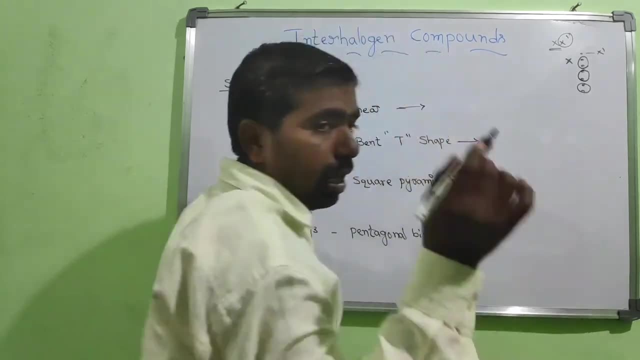 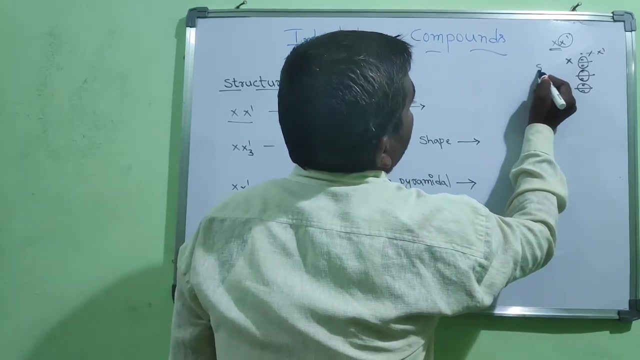 So that is forming with the use of this electron. So now Another electrons are there, So they are. I am considering as a pairs Now the hybridization. I am saying S, P1.. P2.. P3.. 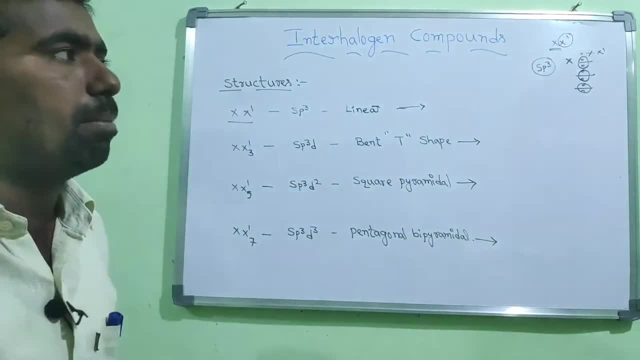 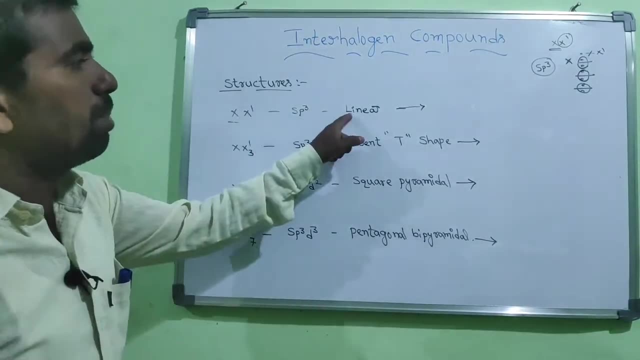 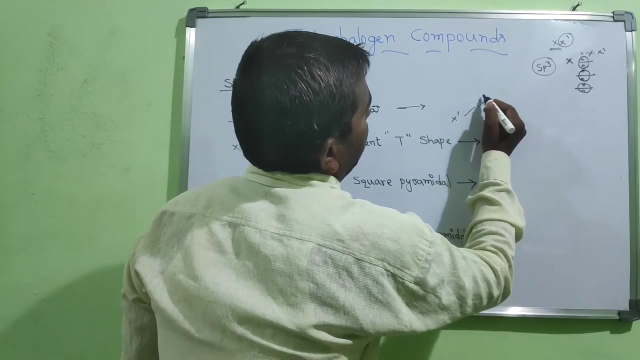 Now the hybridization at the central atom Is undergoing SP3 hybridization. So SP3 hybridization Is occurring at the central atom X, So its shape is linear. So X, X2 dash. There are the three pairs. 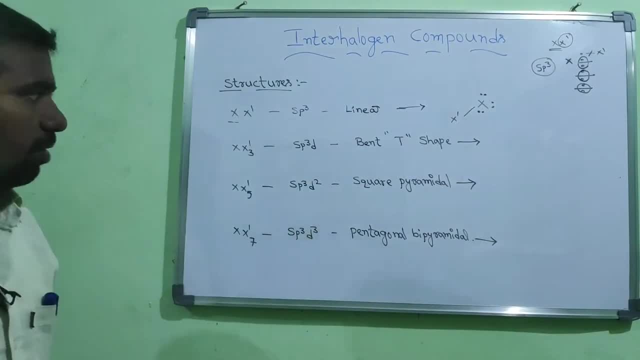 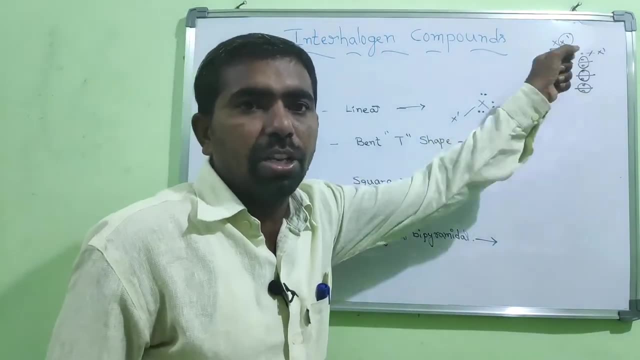 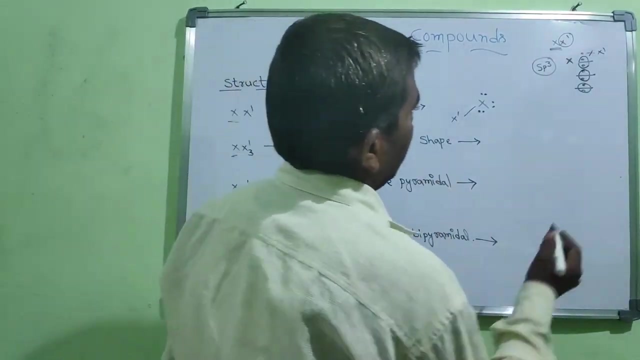 Lone pairs, That is about the structure of XX dash And in the case of XX3 dash. So similar type of Type of explanation, So SP3.. Dehybridization, So molecular shape is the bent T shape. 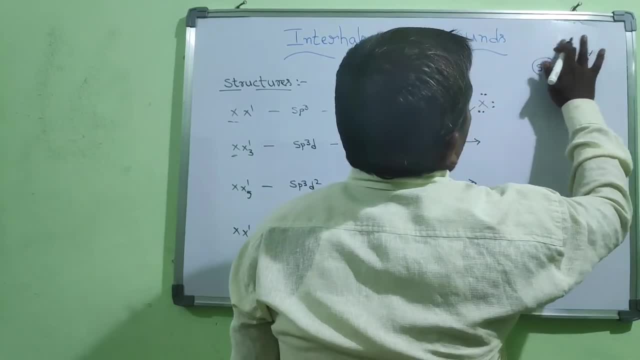 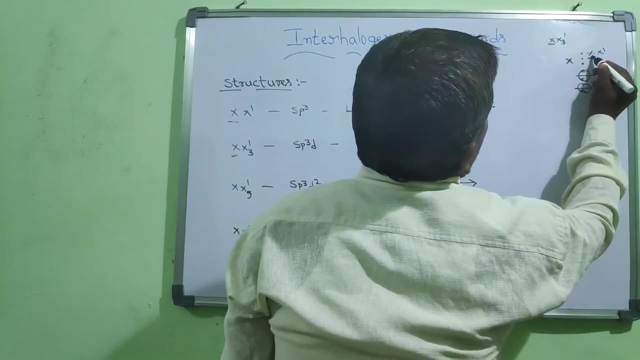 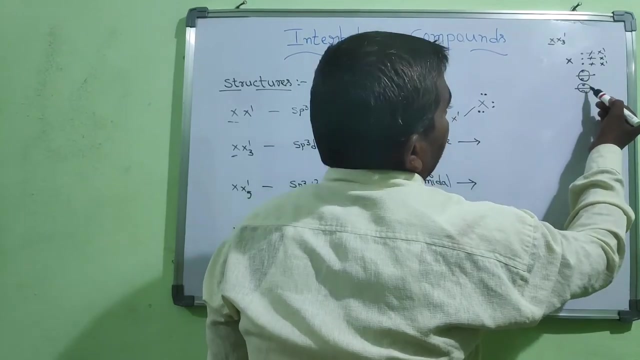 So, for example, XX3 dash I am making here. I am explaining the structure. This is the halogen: 3. Making with the single bonds: S, P1., P2. SP3. SP3D. SP3D is the hybridization. 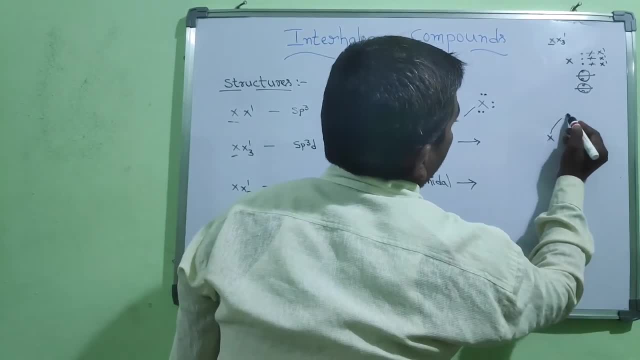 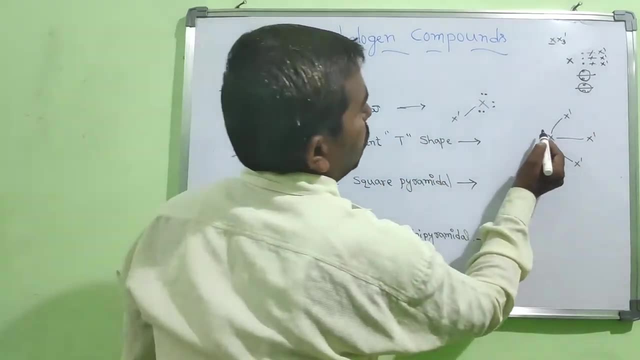 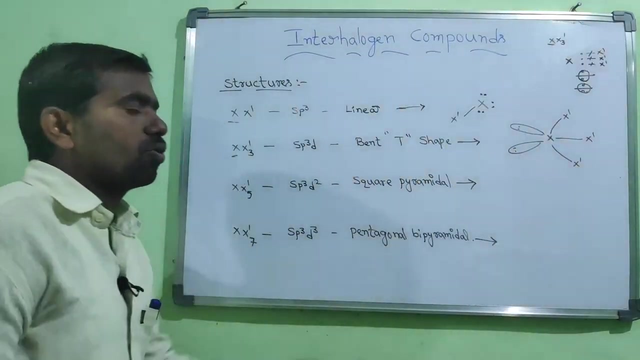 So X is the central atom. So here the X2 dash, Here the another X2 dash, Here the another X2 dash. So remaining two pairs like this. That is the T shape structure. That is about the structure of. 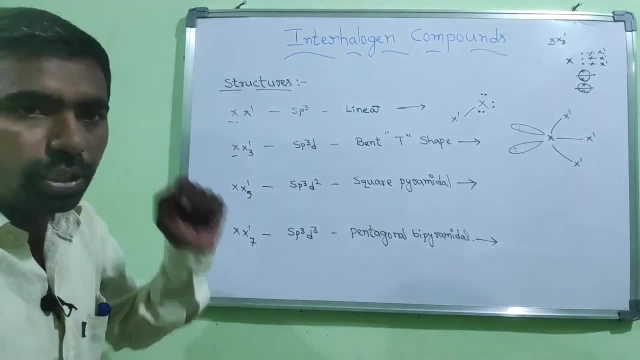 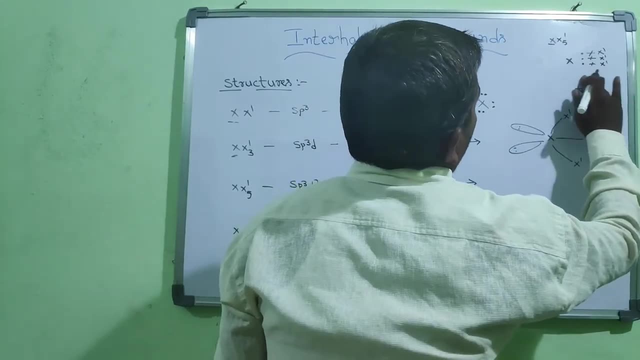 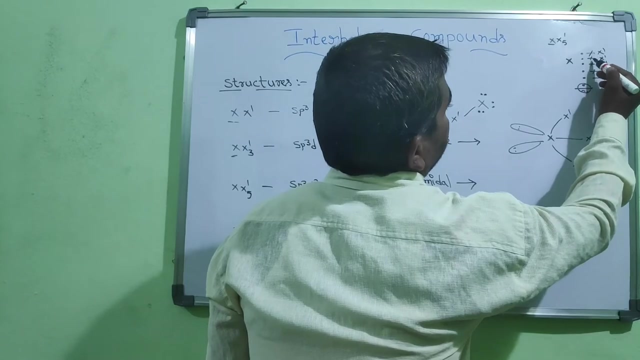 XX3 dash And the central atom hybridization is the SP3D. Now about the XX5 dash. I am taking that molecule here: XX5 dash, So another two halogens. They are making single bonds. Now the hybridization. 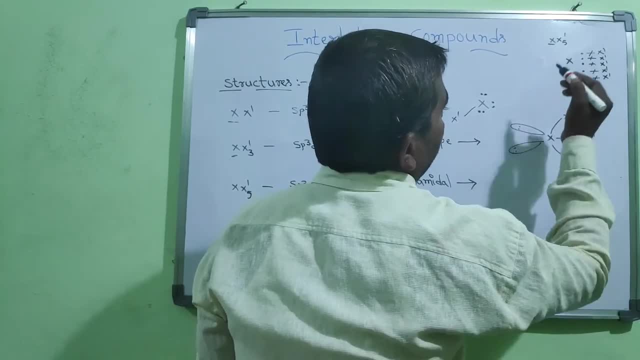 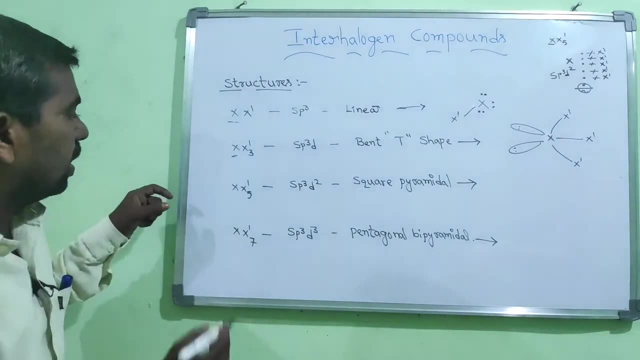 S, P1., P2.. P3., D1 and D2.. SP3D2. Is the hybridization. SP3D2 is the hybridization Is occurring at the central atom X. The molecular shape is the square pyramidal. 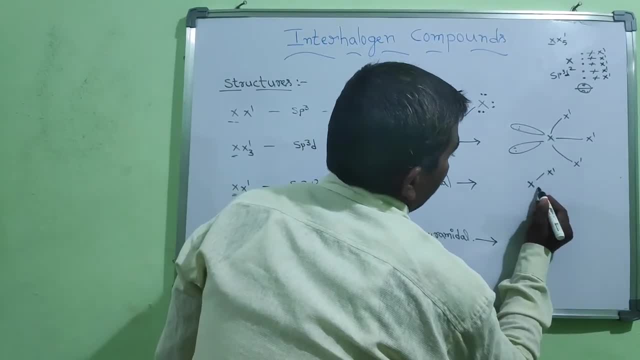 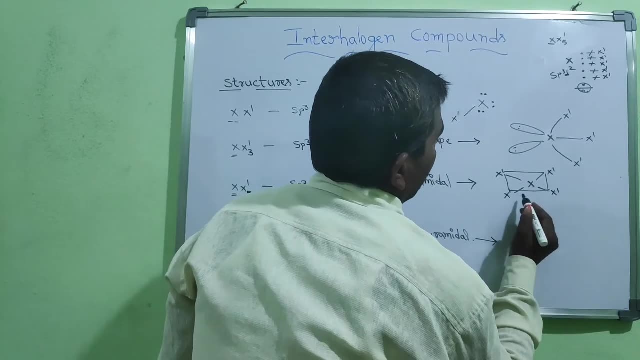 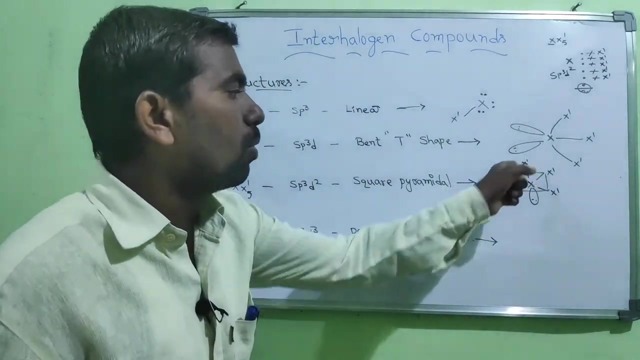 So this is about the X, This is X dash, X dash, Again X dash, Again X dash. This one is the square And one lone pair is there. Another is About the plane, That is about the structure Of XX5 dash. 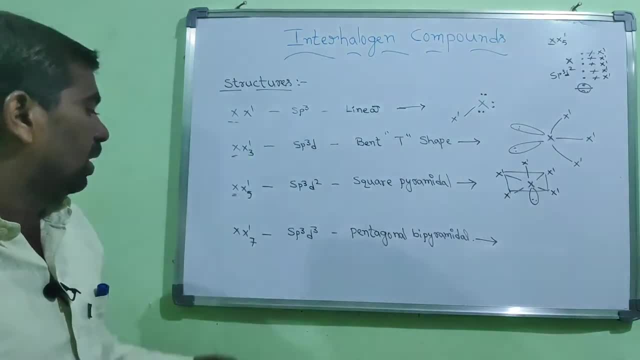 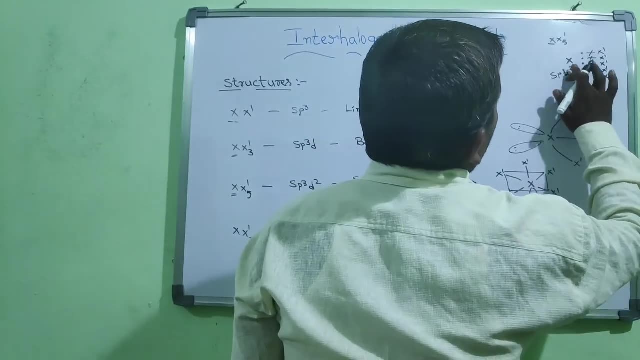 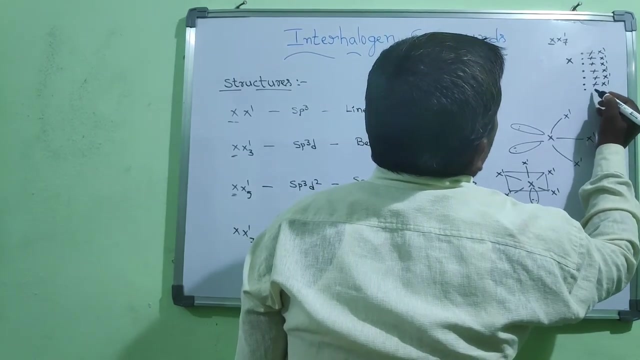 At the central atom. Hybridization is the SP3D2.. Now lost molecule XX7 dash. Hybridization is SP3D3.. That means another two. I am taking XX7 dash- Seven X dashes are there- And making with single bonds. 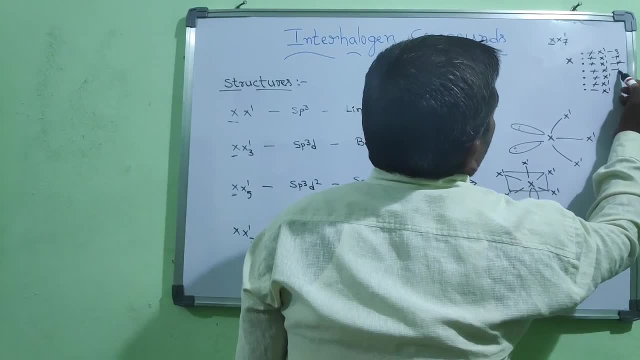 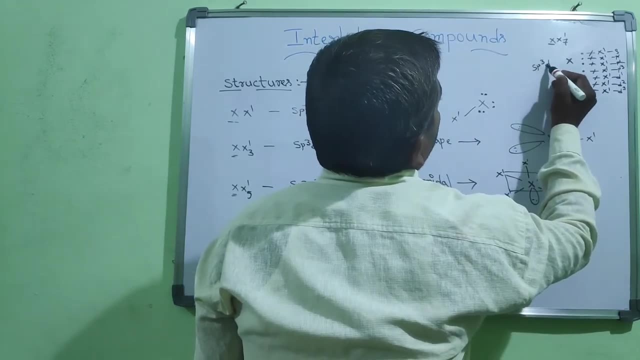 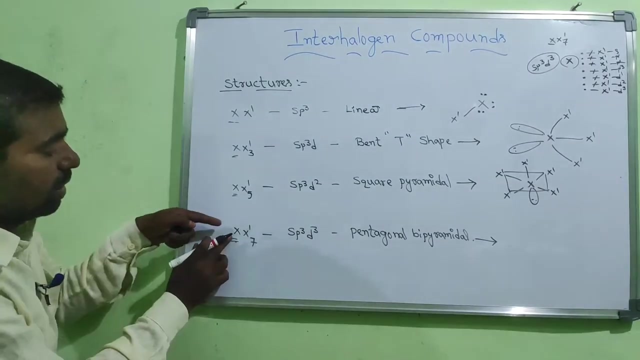 Now the hybridization S: P1., P2., P3., SP3. And D1., D2. And D3.. Now the hybridization is SP3D3. hybridization Is occurring at the central atom X.